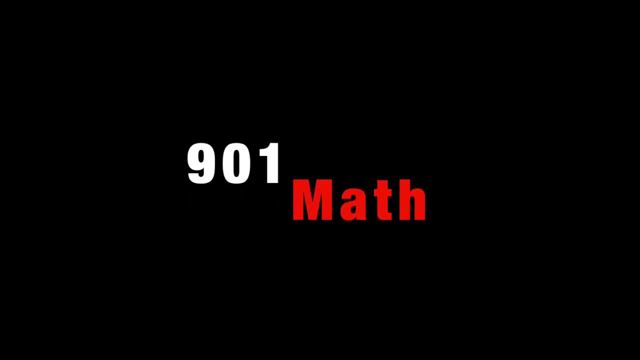 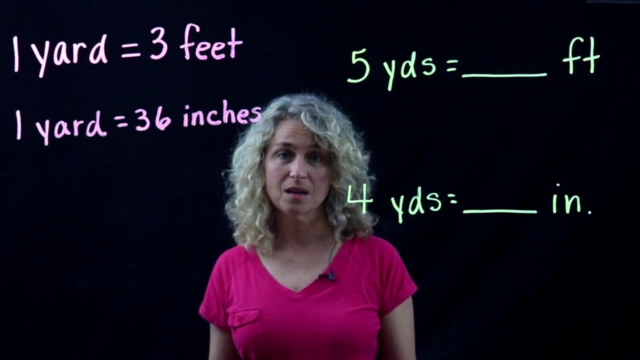 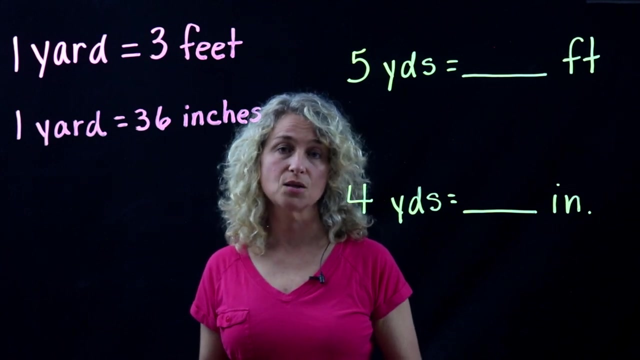 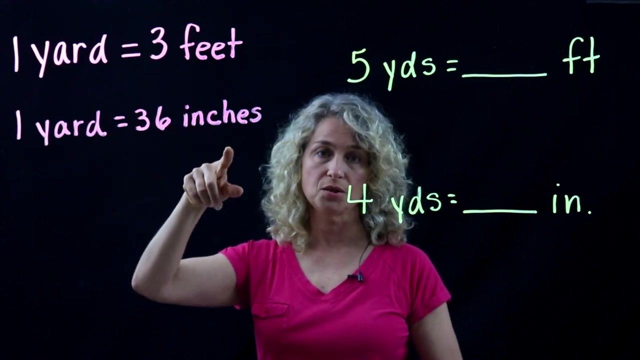 Today we're going to work on measurement and we're going to convert some measurement units. This is with the customary system and these are units of length, All right, so we have yards to feet and yards to inches, So let's look at a couple simple problems. So five yards equals. 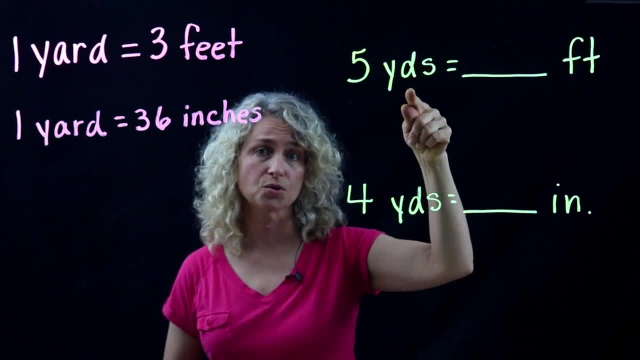 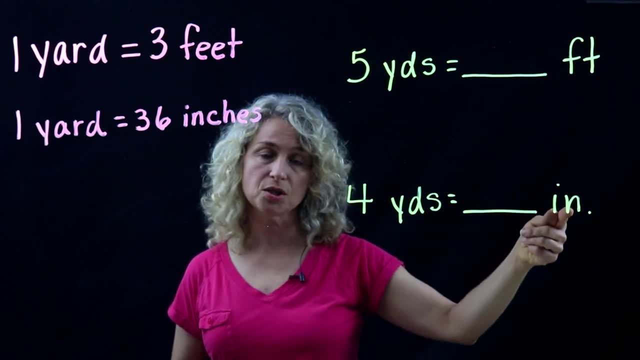 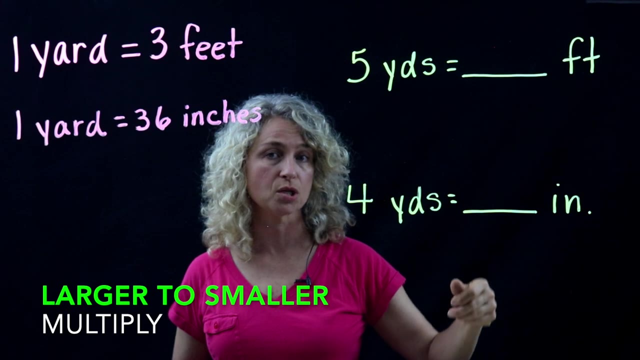 how many feet, If you'll notice yards. yards is your larger unit than the feet. Feet is smaller And yards to inches, this is also a larger to a smaller unit. So both of these are going from larger to smaller. We know we're going to multiply, Okay. 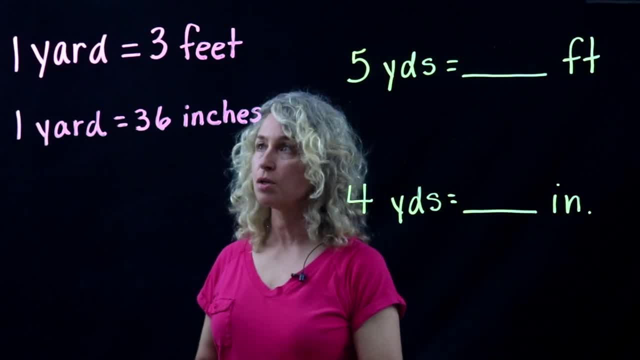 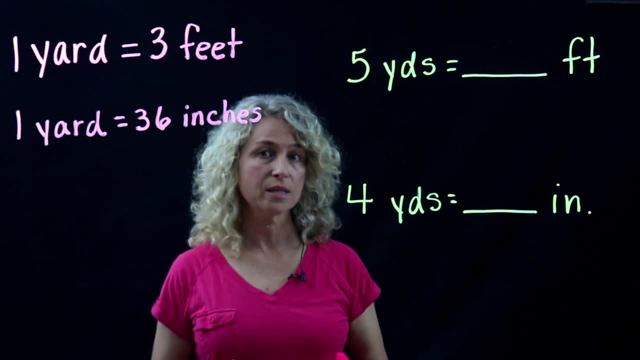 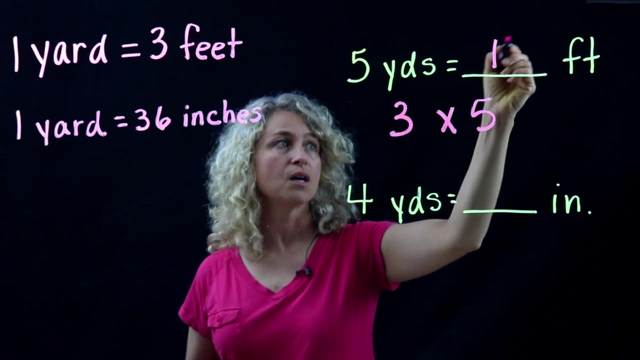 so let's look at the first example: yards to feet, Yards to feet. that is, there are three feet in one yard. So it's simple as that. We're going to multiply three times five and that's it Fifteen. 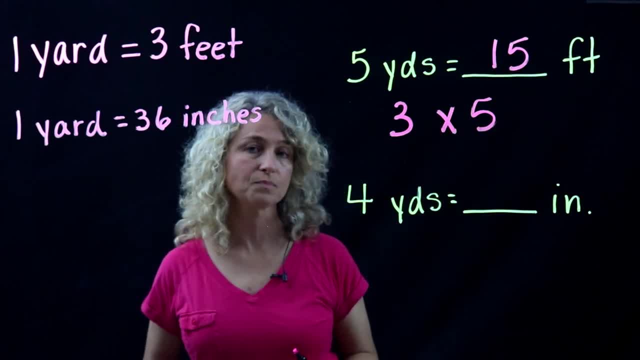 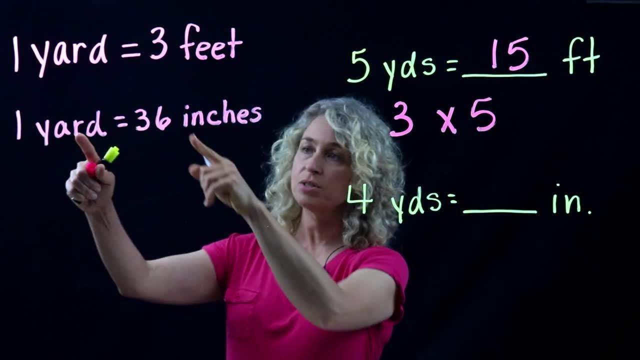 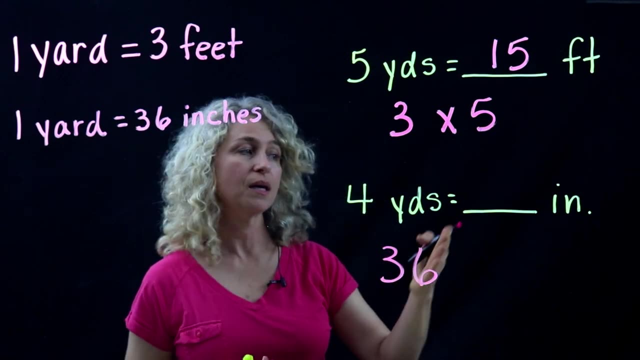 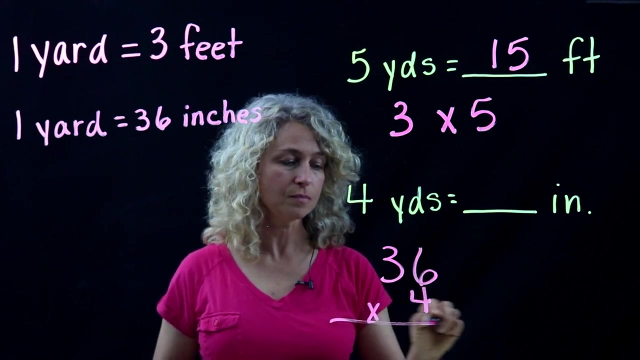 feet are in five yards, All right, so let's look at this next one. The next one is yards to inches, yards to inches. So we have thirty-six inches in one yard. We want to know how many inches are in four yards, So we're going to multiply times four. So when you multiply times four, just do your. 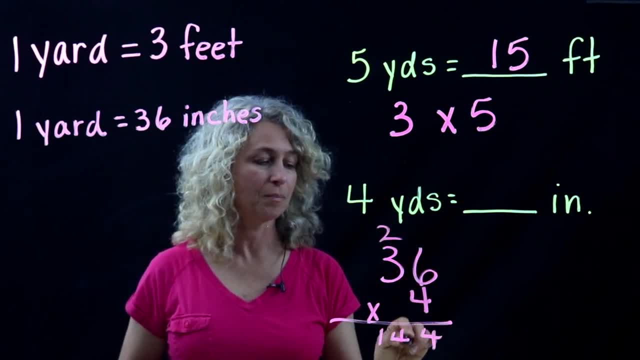 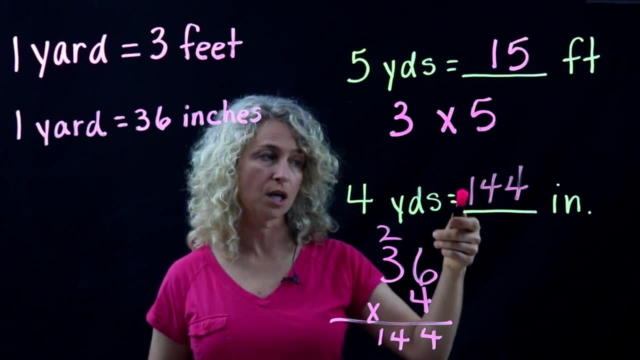 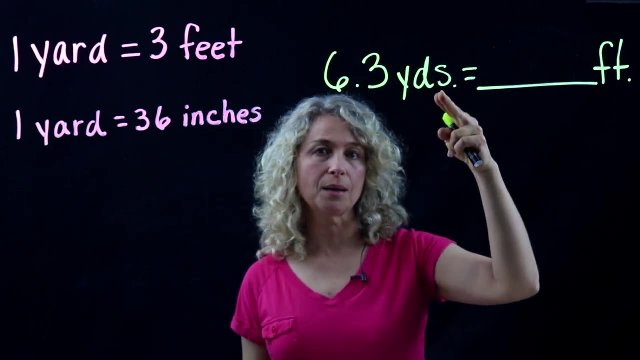 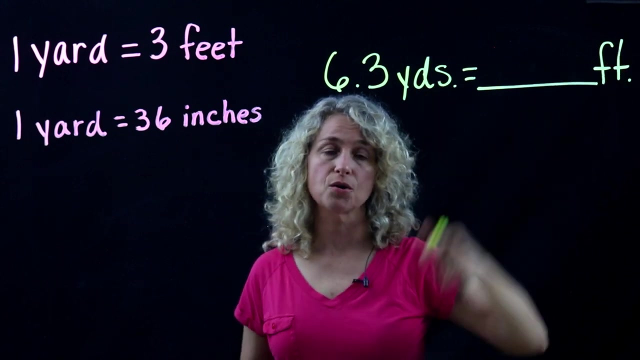 multiplication and get your answer of one hundred and forty-four inches. So four yards equals one hundred and forty-four inches, all right. so if you have a decimal number- 6.3 yards- and you're converting that to feet, you're still moving from yards to feet. that's larger to smaller. you're going to multiply. 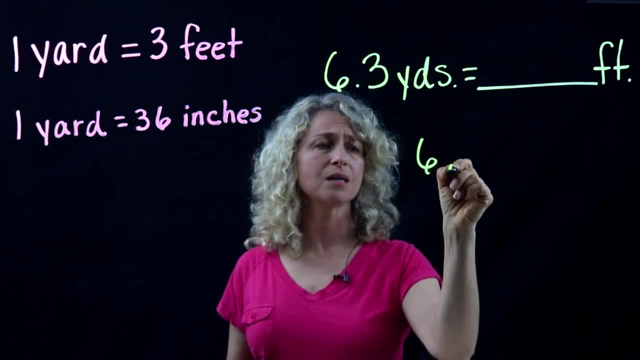 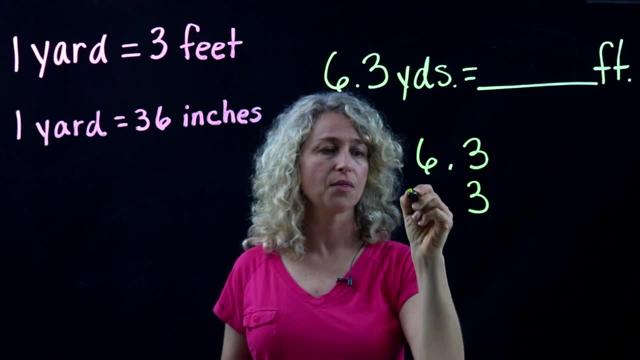 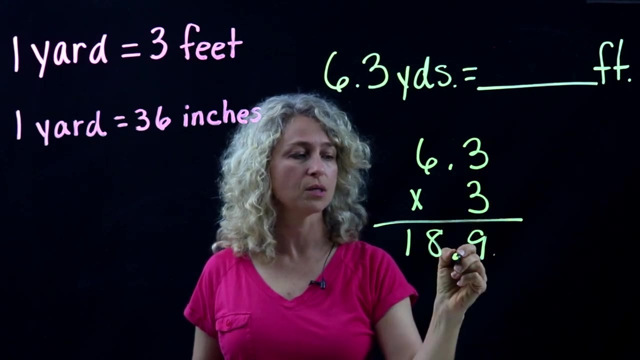 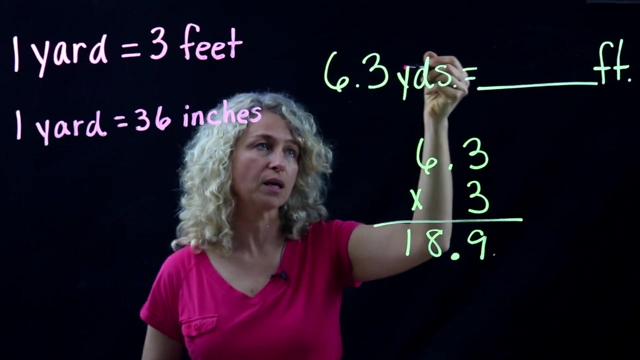 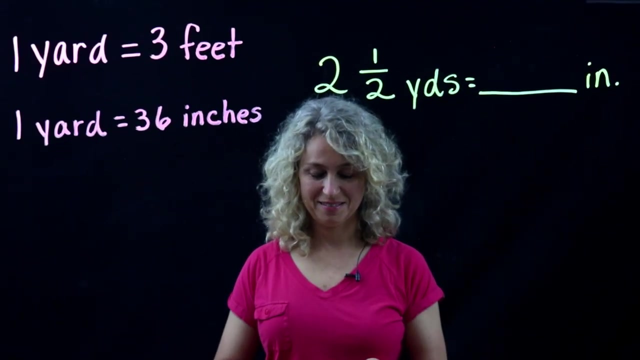 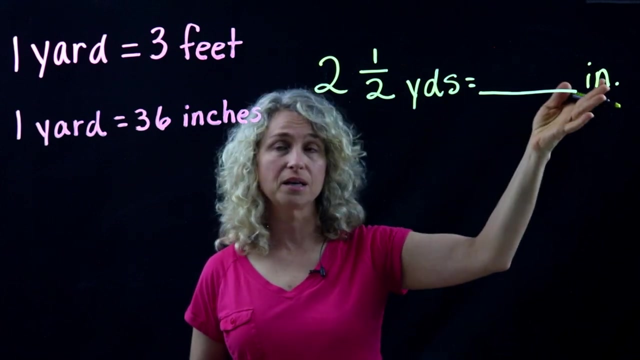 so you will multiply 6.3 times. what well, we're moving from yards to feet. so we're going to say times three and multiply one space over. one space over and 6.3 yards equals 18 and nine tenths feet. okay, all right. so let's look at this one with a fraction: two and a half yards equals blank inches.